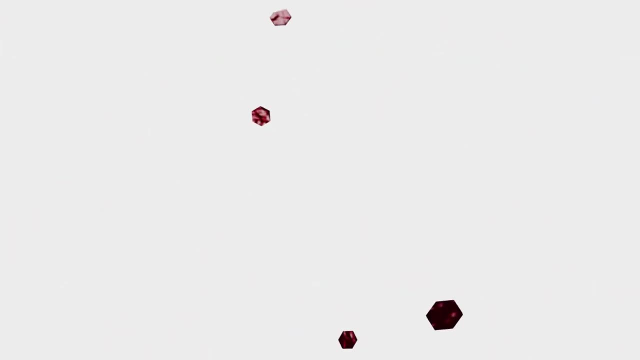 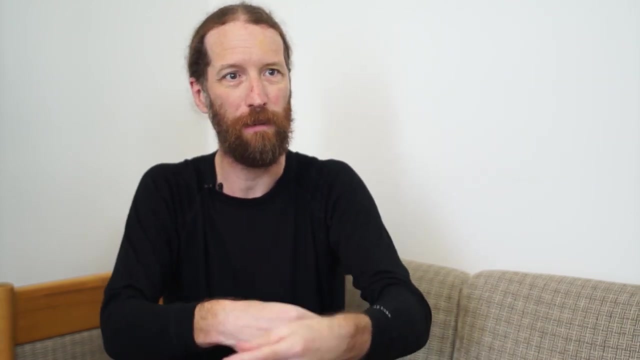 their stick. They break up into really small molecules and those small molecules aren't sticky anymore. It's kind of like tape that's gone old and it won't stick to anything anymore. So it's this very dynamic system. We've developed a framework to describe the sticky behavior. 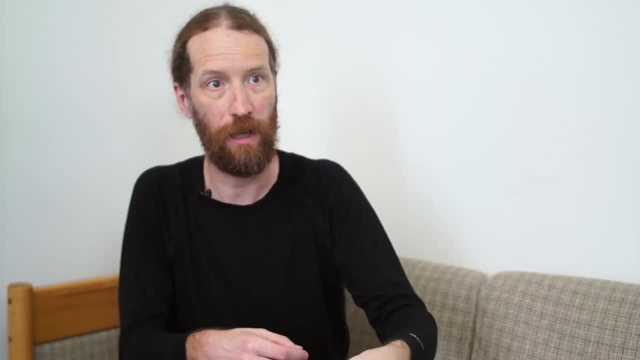 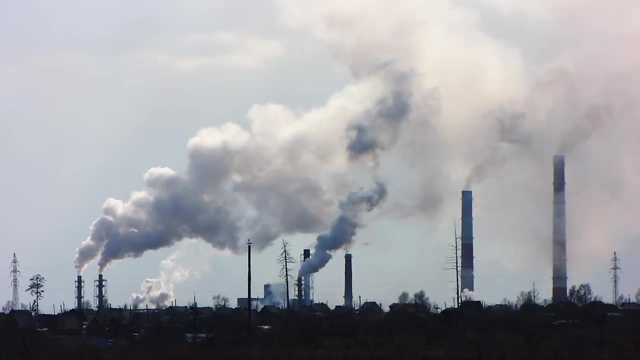 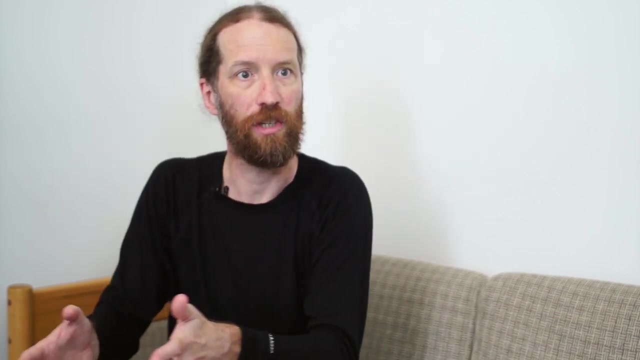 of organic compounds, which we call volatility, which is being implemented in air quality models and climate models. right now. It's already helping to improve the generation of air quality standards, to help improve air quality in states and also in the United States in general, And the implementations in climate models are helping to improve our ability. 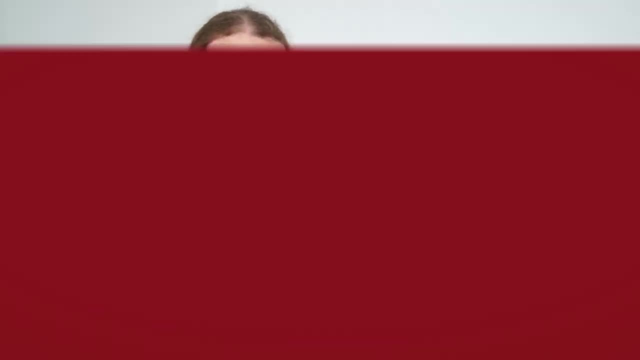 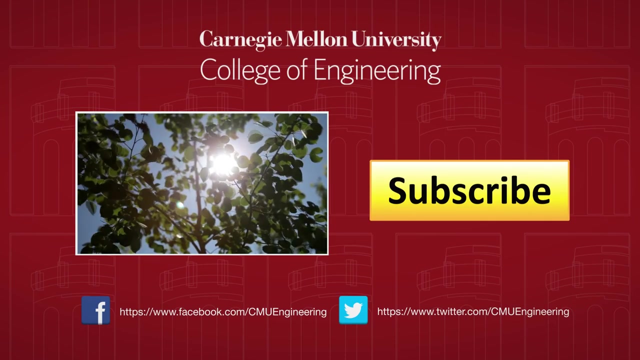 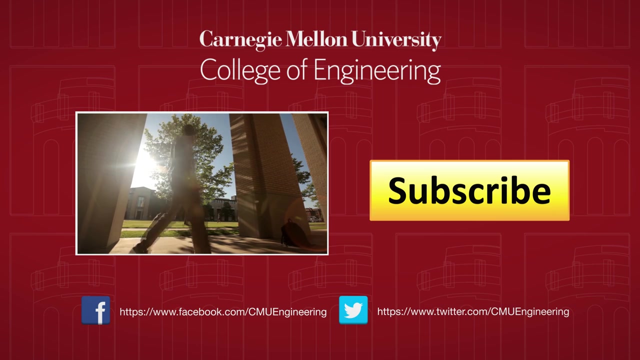 to predict these aerosol effects on climate right now. Thank you very much for your attention and we'll see you in the next video. 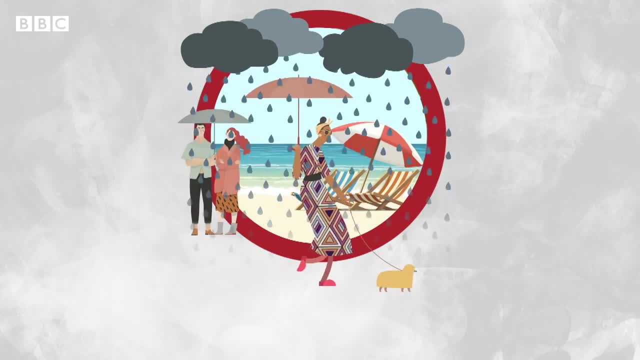 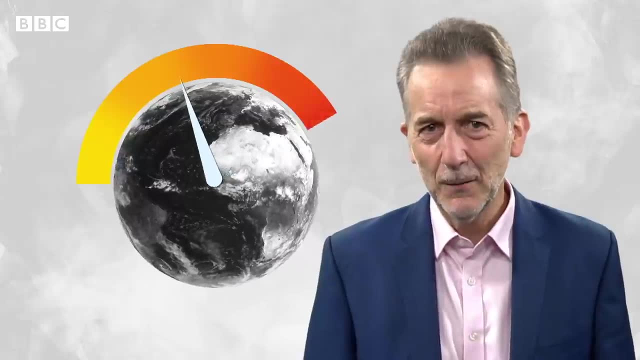 On a cold or wet summer's day, it's not that uncommon to hear someone say: well, so much for global warming. But as our planet heats up- and it really is heating up- it's important to understand the difference between weather and climate. 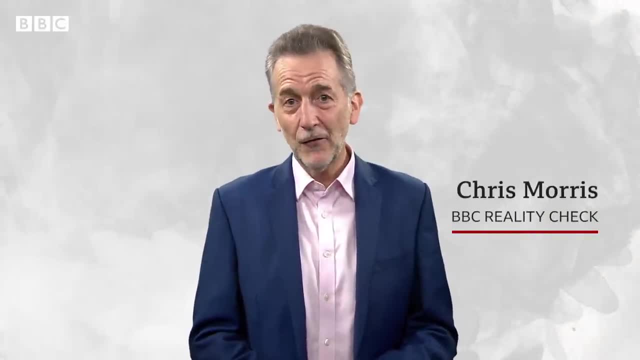 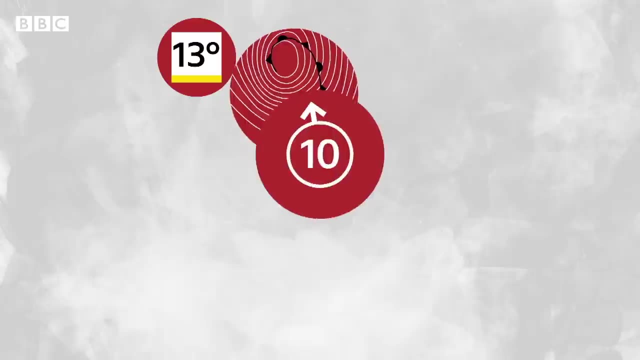 The weather is what's happening right now and how it's likely to vary over the coming hours, days and weeks. Forecasters take a look at things like temperature, air pressure, wind direction and humidity for a particular region. They're all put together into a model which tries to tell us what we want to know. 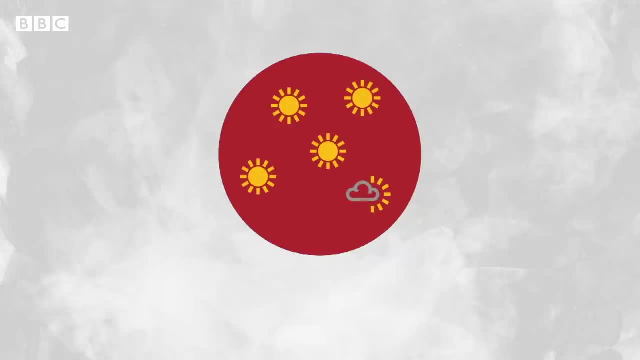 What's the weather like So? will it stay sunny today? How hot is it going to be? When's it going to rain, and is it going to blow a gale tomorrow? What are the chances of a white Christmas? Of course, forecasters don't always get it quite right. 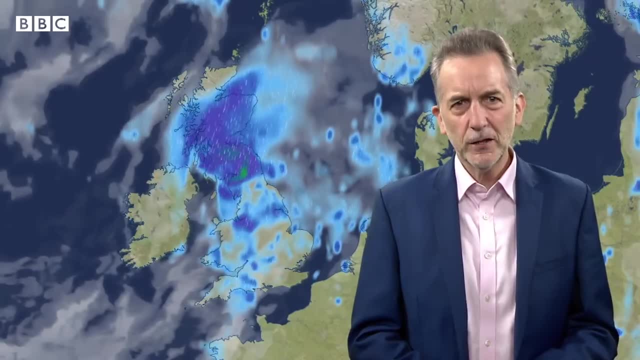 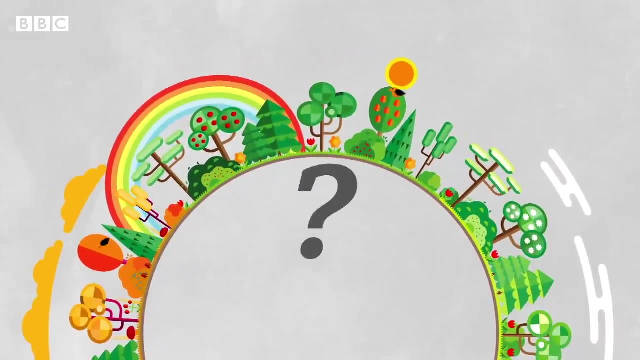 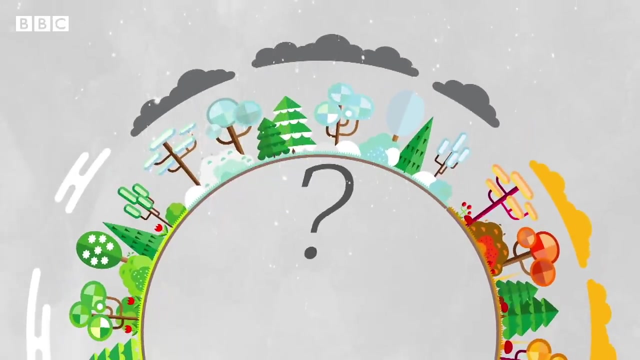 and the weather is constantly changing. But in general, short-term forecasts are pretty accurate for the week ahead. Longer-range seasonal forecasts: Are we expecting a particularly hot summer or an unusually cold winter And more likely to get things a bit wrong? But they are still dealing with the weather and not the climate.